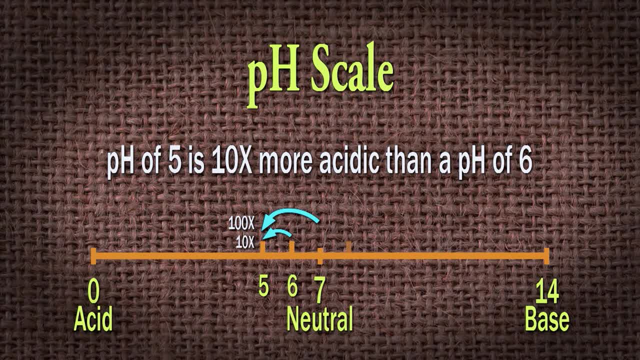 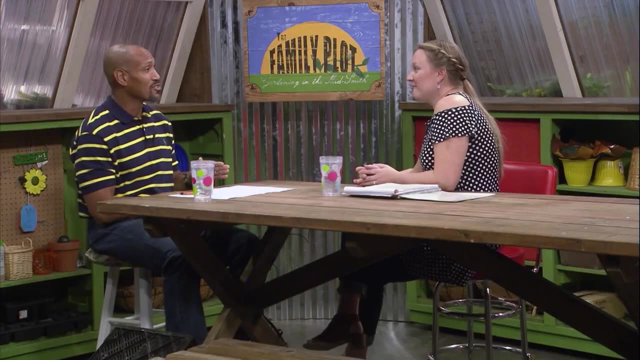 100 times more acidic. So every full single number that you move up, you're moving exponentially. So it really does make a big difference And it's important for us to know what we're starting with so we can adjust properly, Exactly, And I'm glad you mentioned that because people think it's so easy, because they see 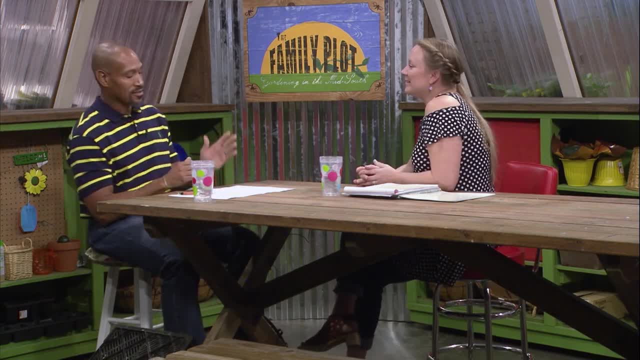 the one number? Yeah, Five to six. Oh, it's just one, Yeah, Right? so, Or even, you know, you're never really gonna get a pH that's more acidic than a pH of six, Right? You're never really gonna get those even numbers anyway. 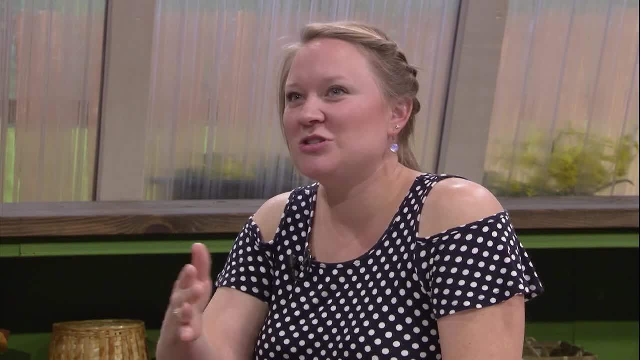 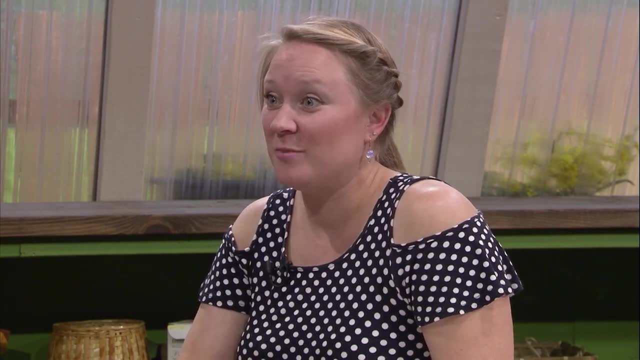 Right. You could get like a 5.4. Sure, Or a 6.2. Right, Or something like that, And they'll think: well, there can't be that much difference between a 6.0 and a 6.5.. 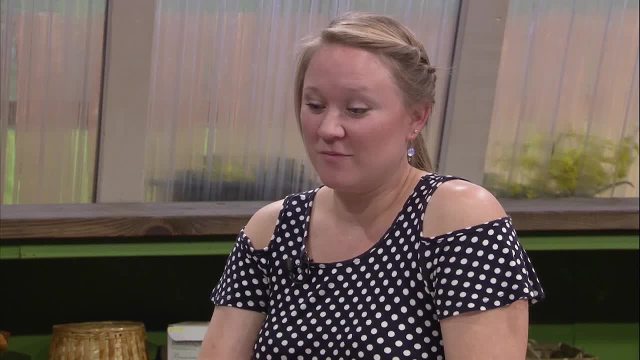 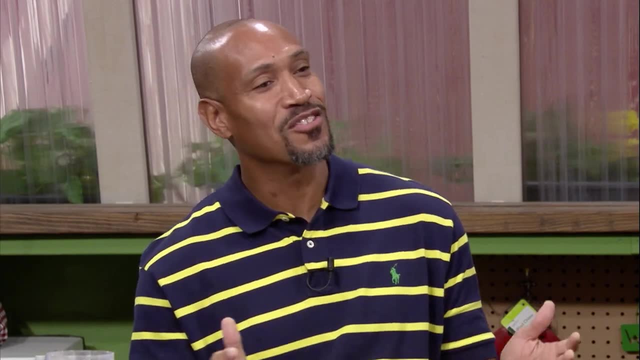 But again, even those decimals need to be taken into account when you're thinking about the exponential scale. All right, Good stuff. So what causes an acidic soil, though? Well, there's lots of different situations. Okay, So in West Tennessee, a lot of soils are naturally acidic. 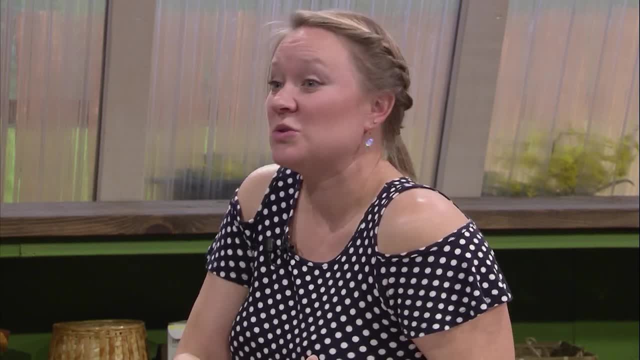 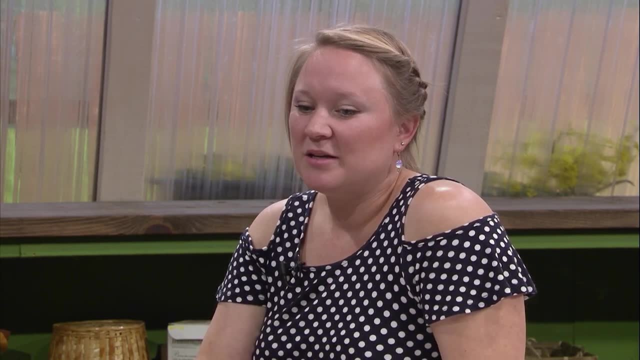 Mm-hmm, And that is just determined by the parent material that your soil is made out of. So, like the bedrock that you know was degraded and now has become your topsoil, a lot of it is dependent upon that. 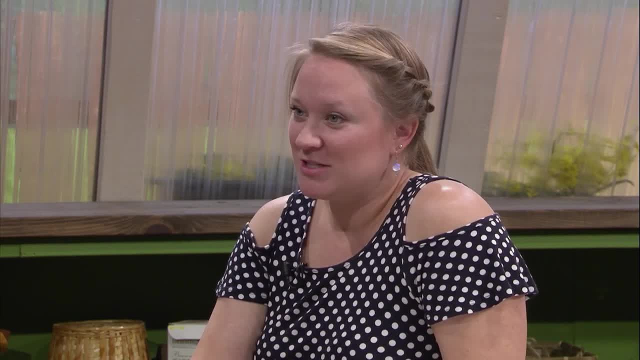 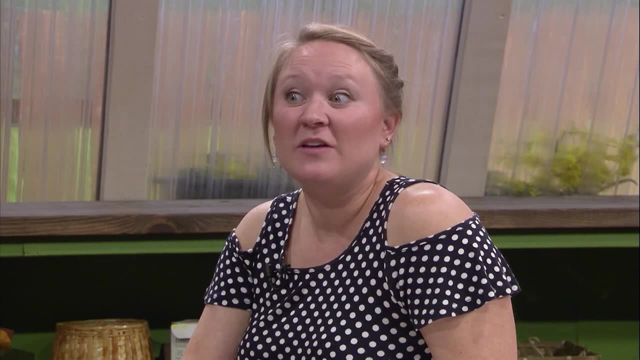 There are also some practices that humans do, so that could create acidic soils, Right. So let's think about there's lots of development going on, Yes, And so anytime topsoil is removed, you're removing some of the Yeah, Yeah, Yeah. Some of the natural amendments of the soil and you could end up with a more acidic soil. New homes lots of times when they remove that topsoil and then they're back filled with what they think might be topsoil, but it isn't really. 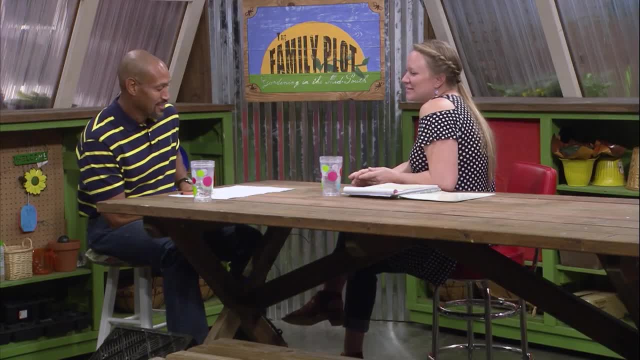 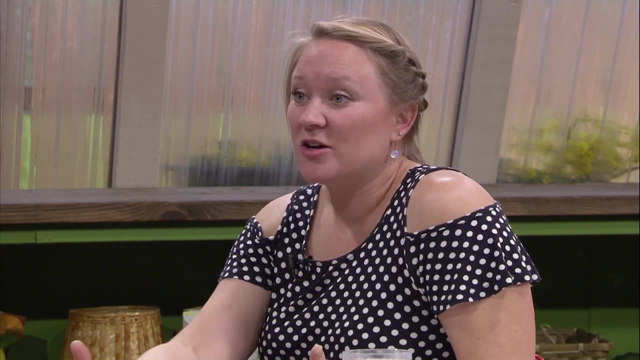 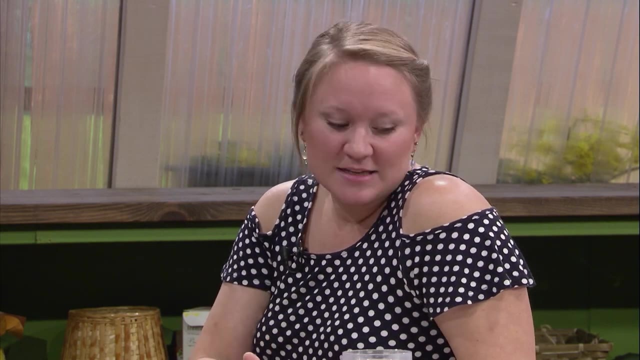 And so, Yeah, Not exactly Right. Right, They could end up with acidic soils that way. Also, just continued use of land. Mm-hmm. Plants are taking soluble nutrients out of the soil, So things like, you know, potassium, magnesium, calcium, and when those are removed from the soil solution, or even removed from water if you're having lots of rain or something like that, those can be replaced with those hydrogen ions, which increases the acidity of your soil. Okay, So any kind of land that's in continuous use might have the potential to be low. have a. low pH or have a more acidic soil. Okay, All right. so what are the benefits of sampling in the fall, though? Right, I mean because you can sample any time. Yeah, yeah, Correct, But the fall just tends to be a little better, you think. Yeah, I think You can sample any time of the year and you can amend any time of the year, But for me, most of the time, especially if we're talking about vegetable gardening, you know where. we've got to have some forethought with this. You want to start a new site in the spring, or you had problems in your garden- It's like this past year- and you want to try to get ahead of the game Sample. in the fall, the lab is usually slower- It is. 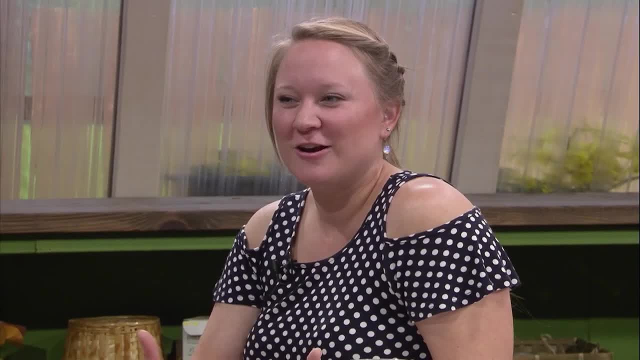 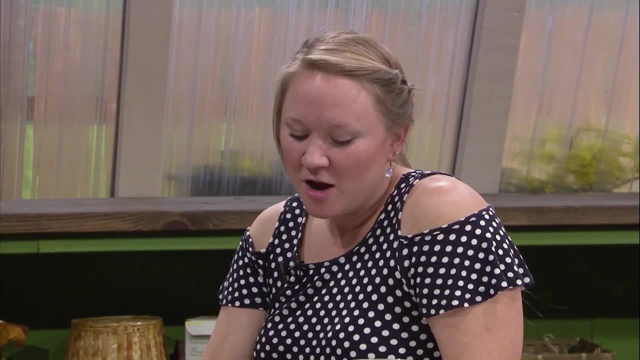 It is in the fall It is Two statements, Because in the spring is when people are getting geared up usually, and so they're sending in lots of samples, So the lab is generally a little slower. you can get your results a little faster. Our soils tend to be drier in the fall, and when you send in a soil sample it really needs to be dry. Okay, If it's not dry when it gets to the lab, then they have to let it dry, So that could add a few days onto your sampling time. And then, of course, if you live in West Tennessee, like we do here in the Mid-South, or in the Mid-South in general, I guess we should say your soils are going to naturally be on the more acidic side. So we're looking at probably around 6 to 6.5, could even be lower, you know, just depending upon where you are. So if we need to amend that pH and raise it, We're going to do that by adding lime, and lime takes time to change the chemistry of. the soil. It's not something that's going to happen immediately, So that's why I like to test in the fall, so you can go ahead and get that lime on the ground now, and by the time spring comes around, you've already started that process of changing. 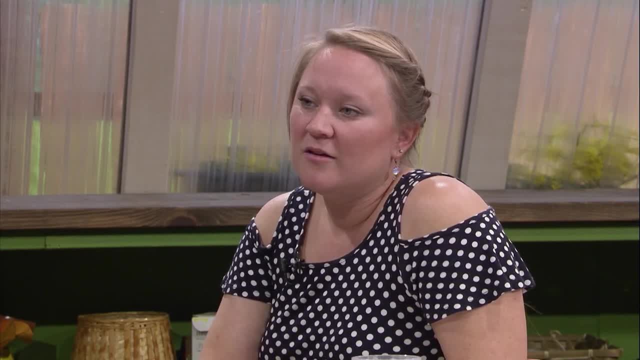 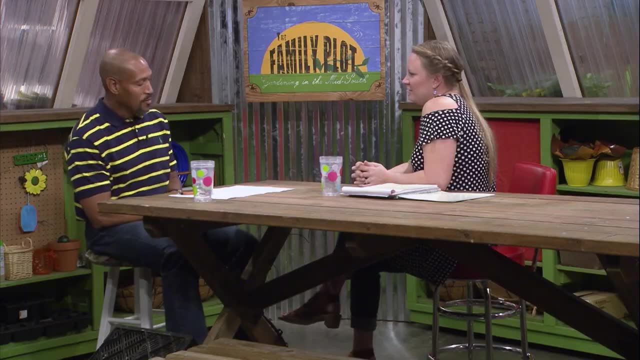 the chemical makeup, So it'd be ready to go for the most part, because it gets weathered in and broken down Right. yes, yes, I've got that, So that's why I prefer fall, Okay, While we have a little time. Lael suggested pH for plantings, though. Yes, What are some of those? Okay, so if we're looking at like lawns, I would say most turf grasses, 6 to 6.8,. I mean you could go a little lower, don't want to go too much higher. They tend to kind of prefer some of that. acidic soils, Okay, Areas that are naturally kind of like wooded- Okay. If you have a wooded lot around your home, those soils are going to be naturally more acidic because they're having a lot of leaves and things that are falling and decomposing. so that would be common, you know, for that type of area, Gardens, vegetable gardens, in general. again, we're looking at probably 6.0 to 6.8, somewhere around that area Where you want to really make sure you have more extremely acidic soils would be for crops. like blueberries? Yes, So there you'd be looking at like 4.8 to 5.2.. Yes, Man, low. Yeah, so if you test an area and you're not sure what you want to do with that piece of, your property and it comes back low in that range, maybe you would want to plant blueberries there, because then you don't have to fight with amending that pH, because pH doesn't stay changed. Right, You know, you have to stay on top of it and continue to amend it if you want to move the 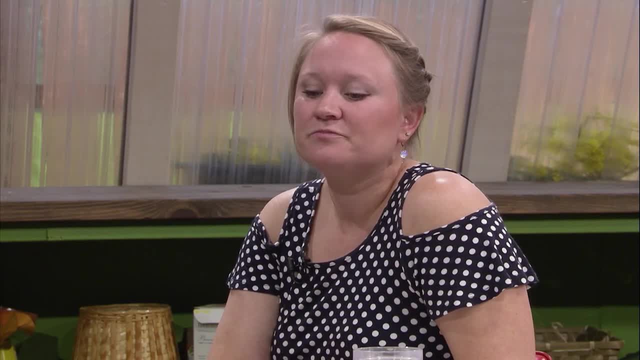 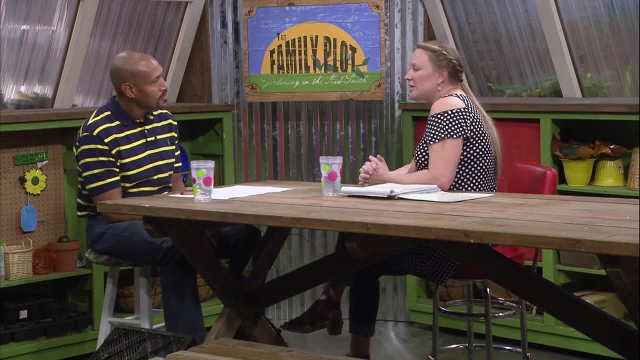 natural. Yeah, level of that pH of that soil. Okay, Well, since you're there, let's quickly talk about how do you adjust the soil pH there? Oh, okay, definitely. So we can really only know amounts if we get our soil sample, like how much we need to. add. So that's another reason why it's so important. If we're wanting to raise pHs nearer to seven, you've got an acidic soil and you need to raise it nearer to seven. you're going to add lime? Okay, All right. 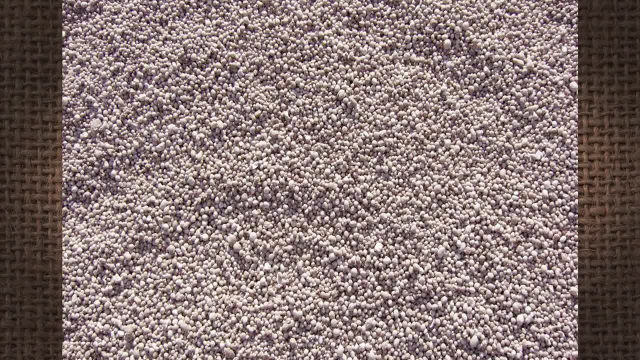 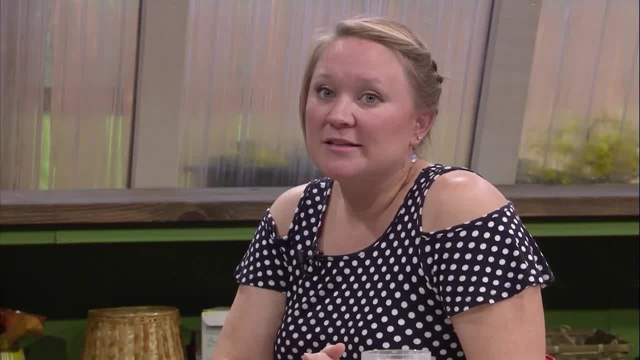 For homeowners, pelted lime is going to be the product of choice. Sure, It's going to apply, but then again, you know it takes time to do its thing. Okay, We, I would not put more than 50 pounds per thousand square feet out at a time. 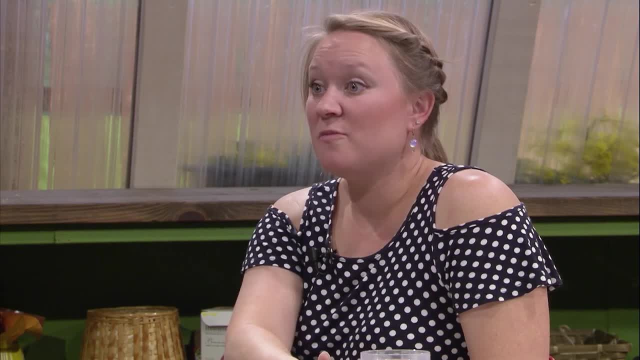 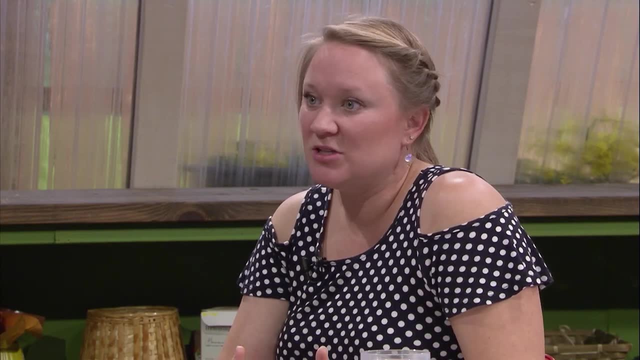 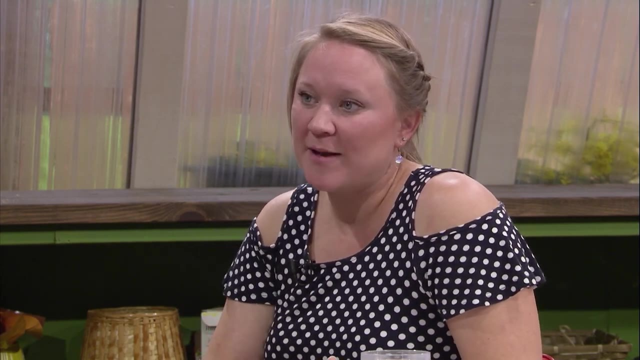 Interesting. Okay, Because there again you may be getting a lot of waste if you over apply. If you put 200 pounds out, it's not all going to be able to do its thing Right, Gotcha, Gotcha. So sometimes if we have a drastic adjustment, you may have to split up that application. into two or three applications throughout the year. Okay, So apply the first one now. wait two or three months, apply it again. wait two or three months, apply it again. Makes sense. And then retest. Okay, To see where you've gotten yourself to and how much more you need to go from there. If you have. if you're trying to go the opposite way and lower your pH, say that you have a spot that tests like 6.8, but you really want to grow blueberries there, Or you really want to grow some acidic shrubbery there. Plants that prefer acid soils, like azaleas, rhododendrons, hollies, things like that. Adding sulfur can get you down to that lower pH area where you want to be, And that's that elemental. Elemental sulfur can do the job. I probably wouldn't want to use that every single time. Aluminum sulfate will do it as well. So you know either product And it just depends. There. again, you need to have results from your soil sample to know how much you need. to move, But as a rule of thumb, I think it's like .2 pounds per hundred square feet to move it, a tenth of a pH point. So it's, you know, gonna take some calculations and some time, but we need to know what we're. 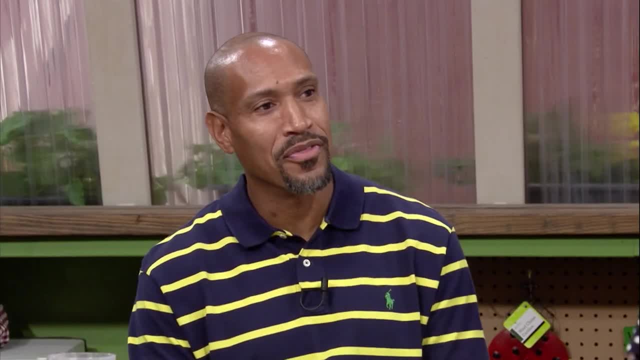 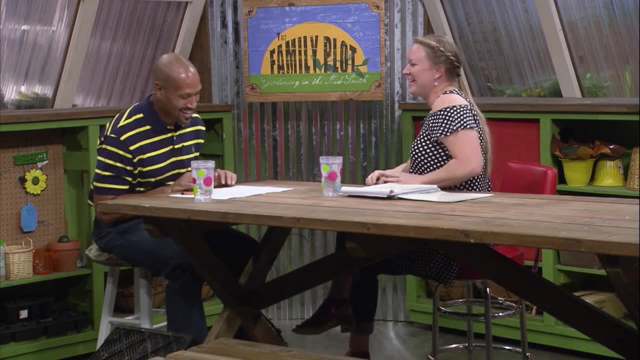 starting with before we start adding: Wow, Garden math. I know garden math. How about that? I'm always bringing math to the scene. I'm always bringing math. We're glad to have you back, The garden mathematician, So you can do the math.